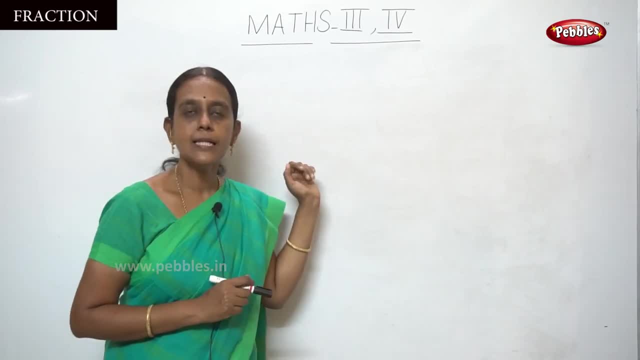 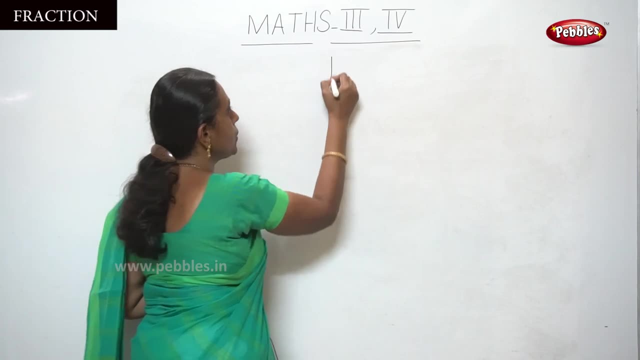 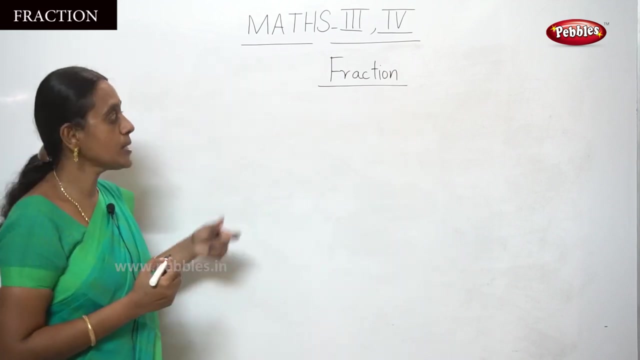 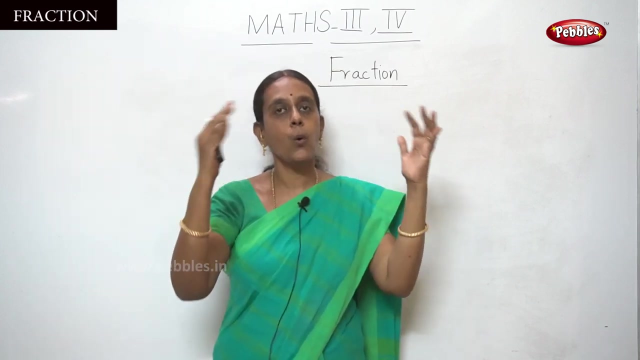 Dear children, today's our new topic is that is fraction. Okay, we have discussed previous topic, that is division. This also fraction is also that is closely related with division. Okay, and what is meant by first? that is fraction, Okay, fraction is a part of whole, Okay, 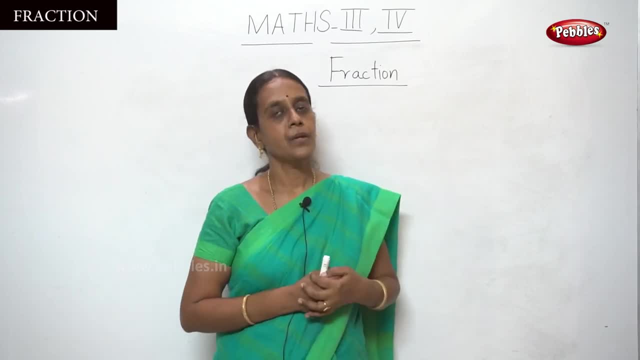 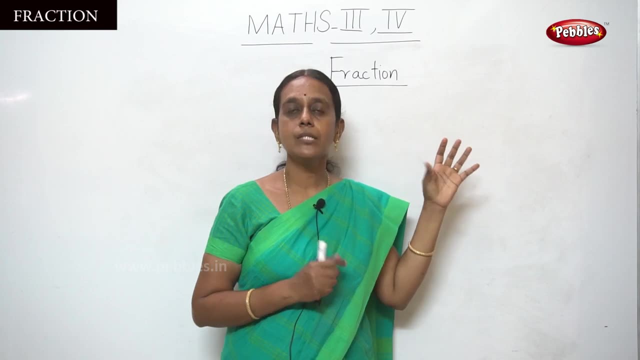 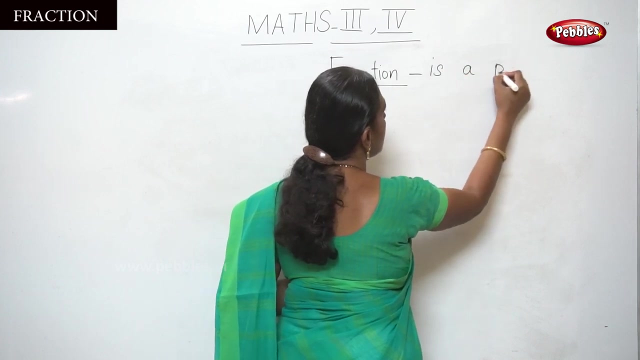 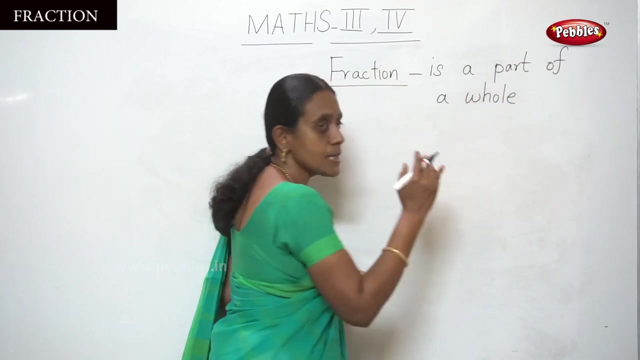 I am going to explain one diagrammatical example. Okay, you can understand easily. Okay, that is fraction. That is a definition for fraction is a part of a whole. Okay, I am going to write the definition: Fraction is a part of a whole, Whole means total. Okay, 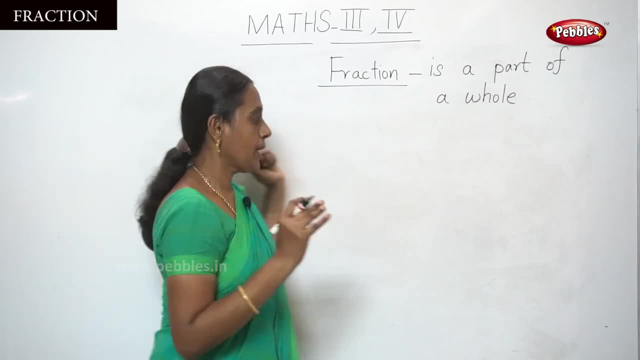 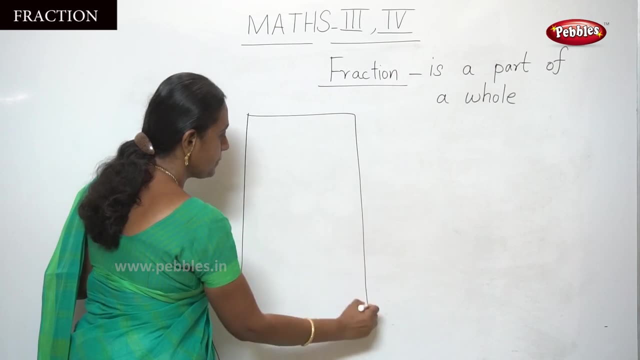 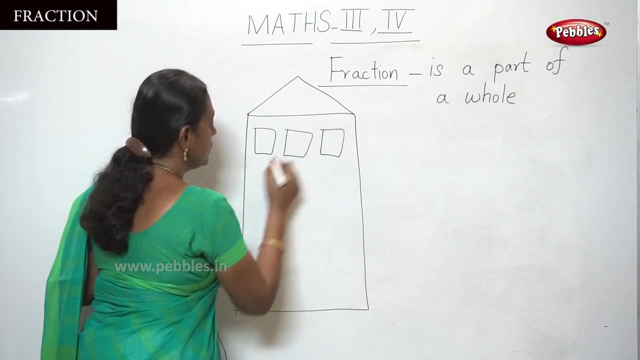 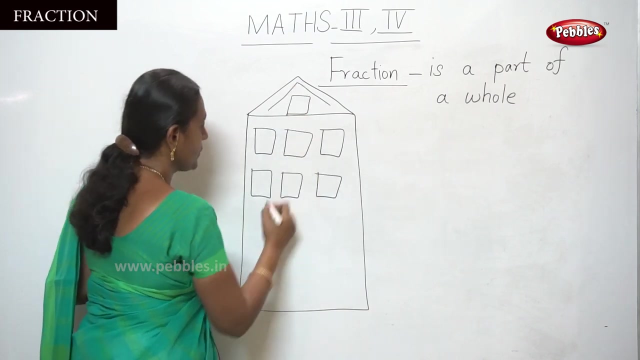 that is a one portion that is called fraction. Okay, let me discuss one example Here. I am going to draw one drawing, Okay, and that is: this is a tall building. Okay, so it is a tall building and it is a flat system building. 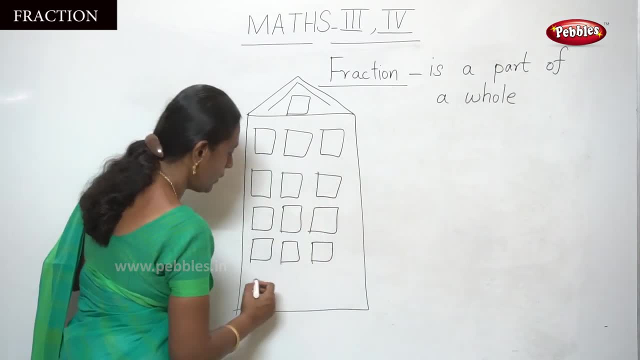 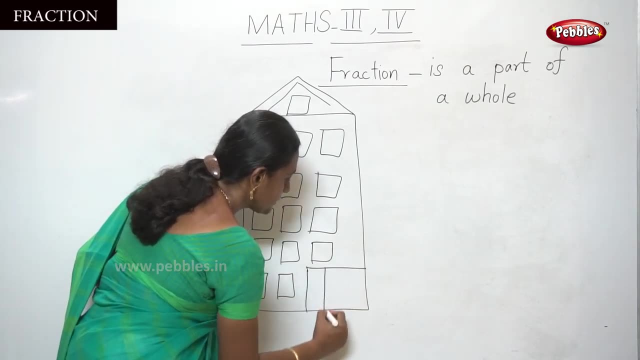 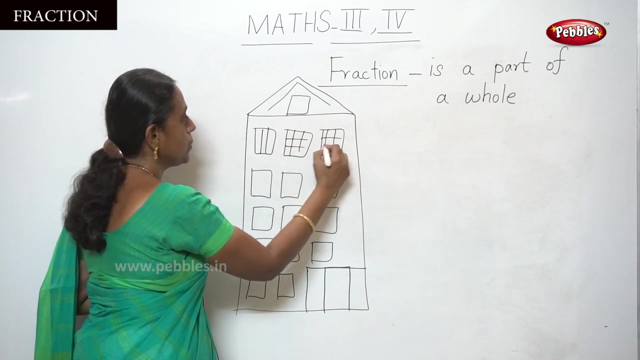 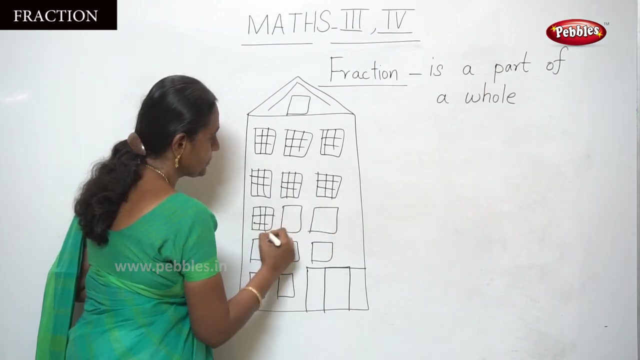 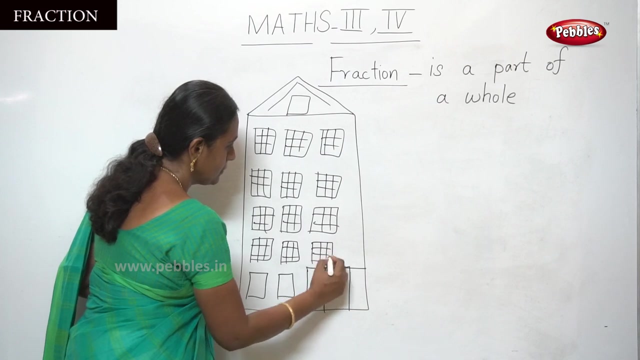 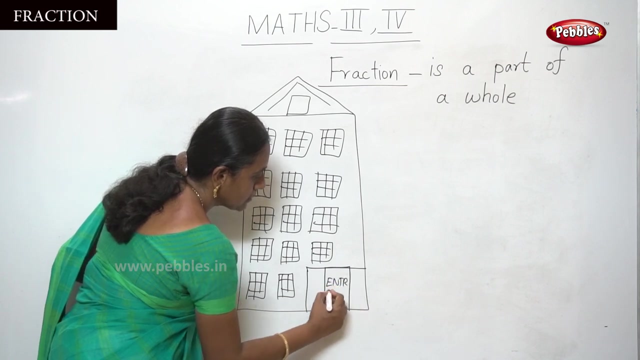 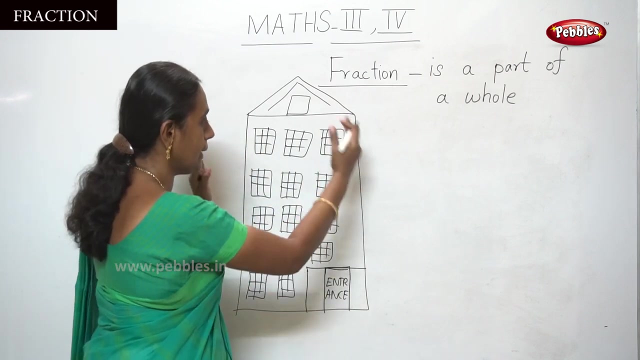 Okay, it has. that is 1,, 2,, 3,, 4, 4 storey building. Okay, and that is Okay. and these are the windows, Those. this is a entrance door. Okay, this is a door. Okay, so this is a long 4 storey building, Okay. 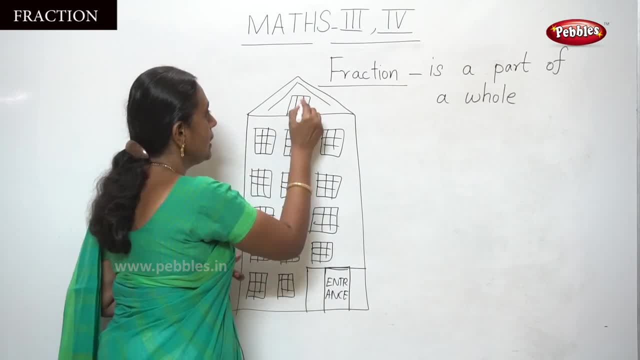 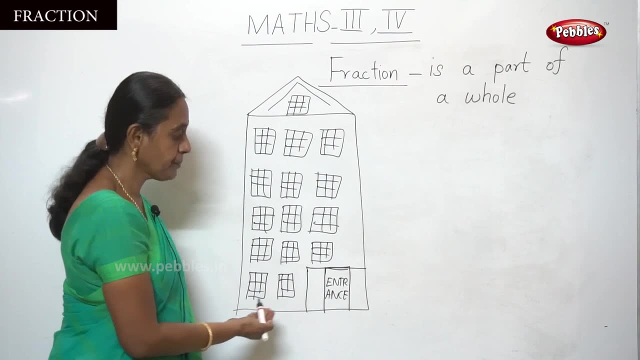 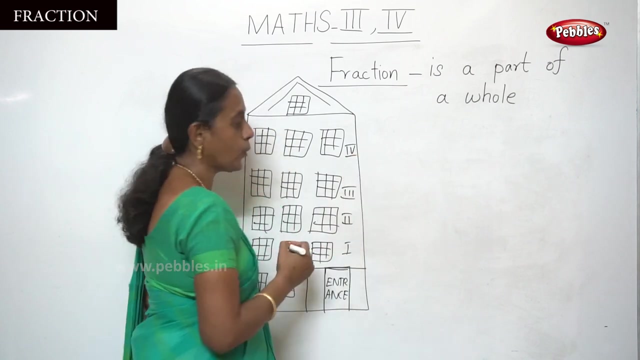 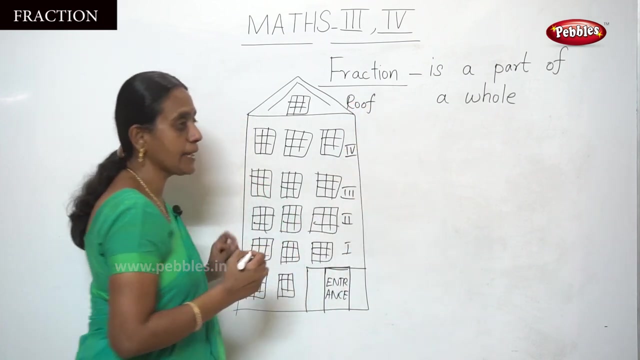 now we can have to calculate the number of, that is, doors in each floor. Okay, this is a ground floor And this is a first floor And second floor, This one is a third floor And fourth Floor And this one is the roof. Okay, So now you are going to write the number of doors and that. 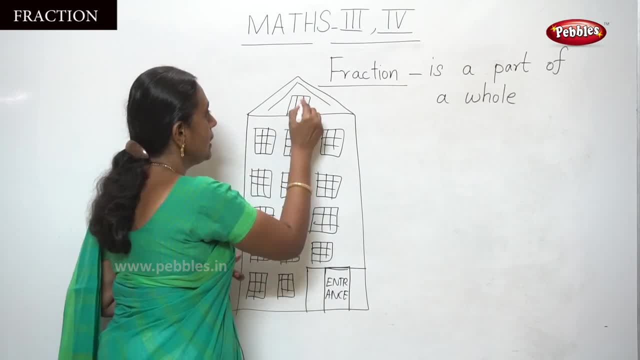 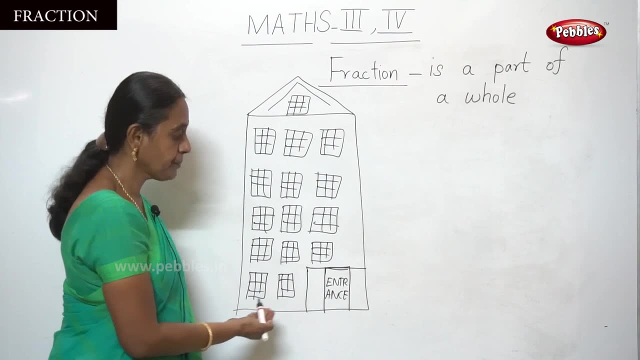 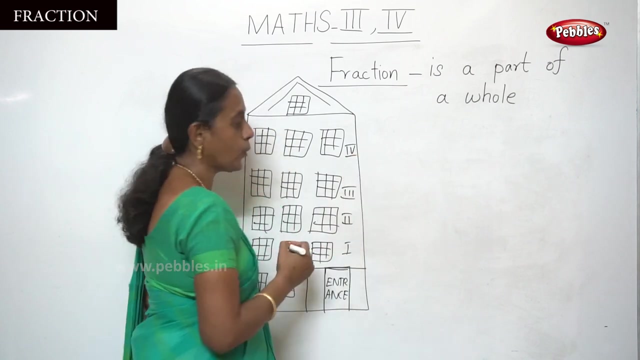 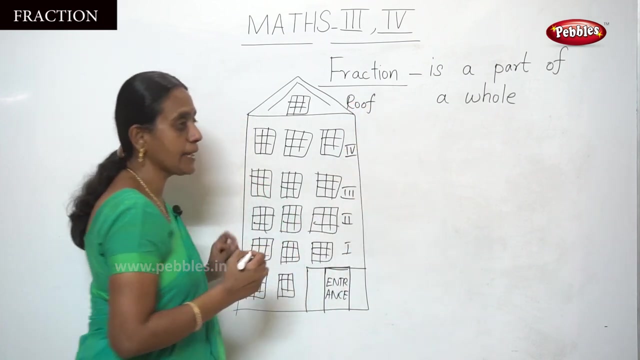 now we can have to calculate the number of, that is, doors in each floor. Okay, this is a ground floor And this is a first floor And second floor, This one is a third floor And fourth Floor And this one is the roof. Okay, So now you are going to write the number of doors and that. 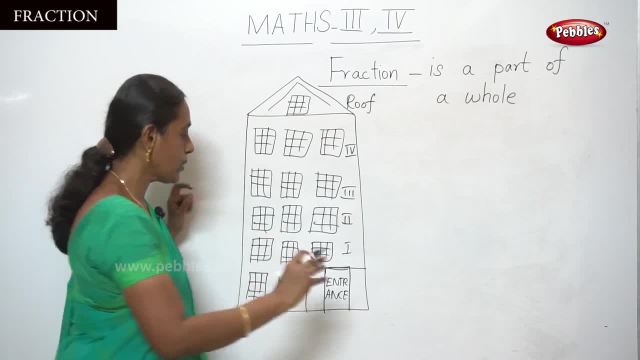 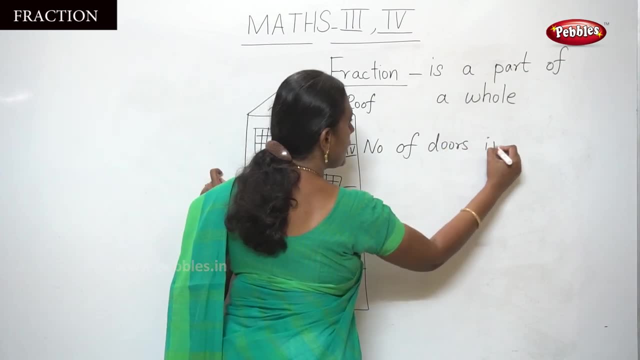 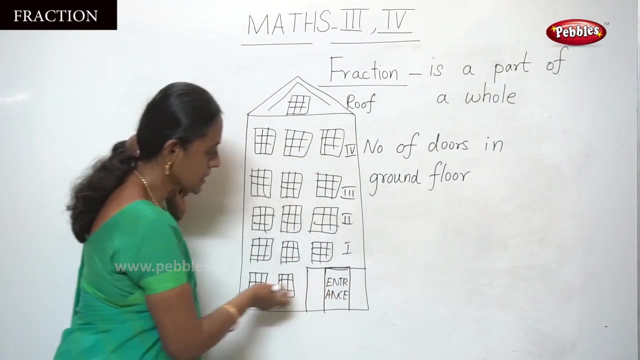 is ground floor. So you have to calculate. I'm going to write the question: Okay, number of doors in ground floor, Number of doors and ground floor. This is a ground floor, And this is a first floor, And second floor And this is a door. Okay, This is a second floor. So 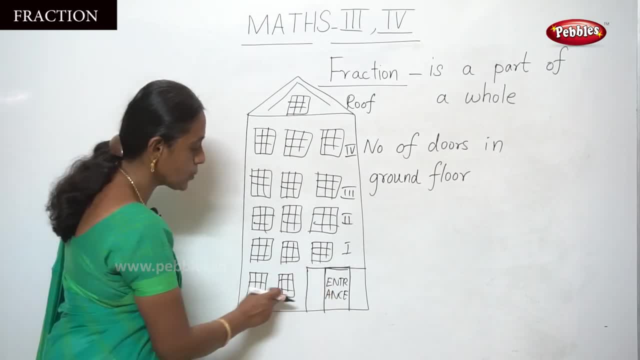 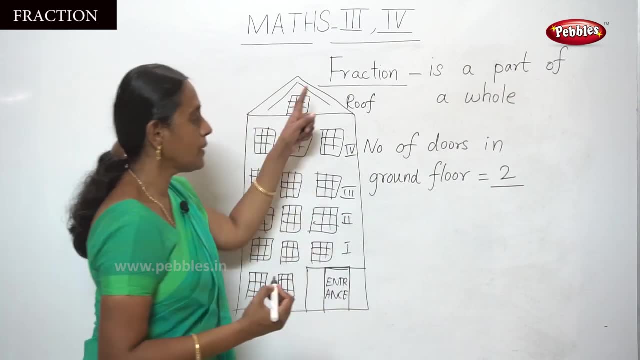 here you have to count the door, that is 1. And 2.. This one is the entrance Okay door. These are the two doors, So that is number of doors in ground floor. That is 2. And fraction is always. 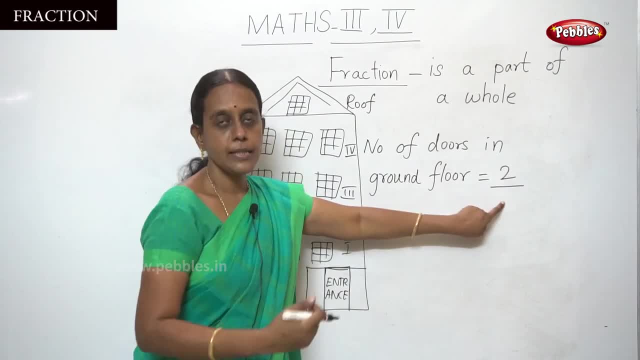 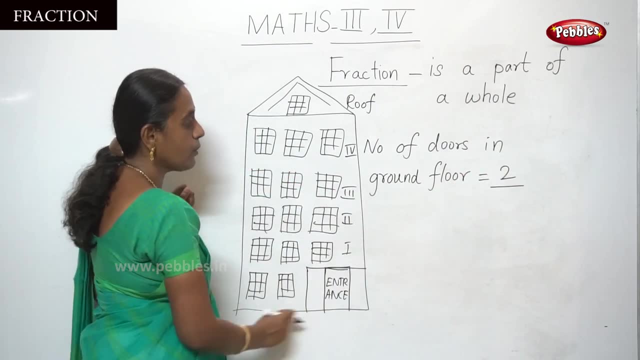 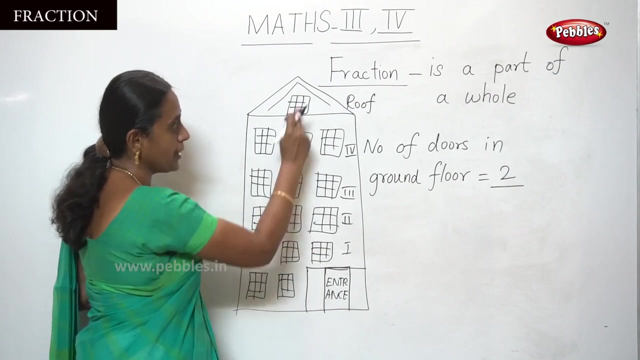 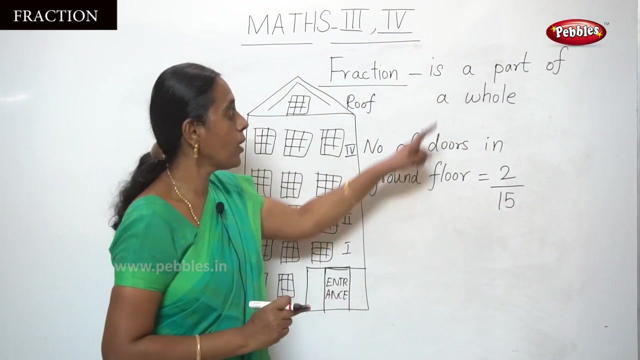 be like this: one number is we have to write and top and the other number, that is, should be written in below. So fraction is like that: two by an other number down. here that is all: 3, 6, 9, 12, 13, 14 and 15. here that is 15. this is a total portion that is called. 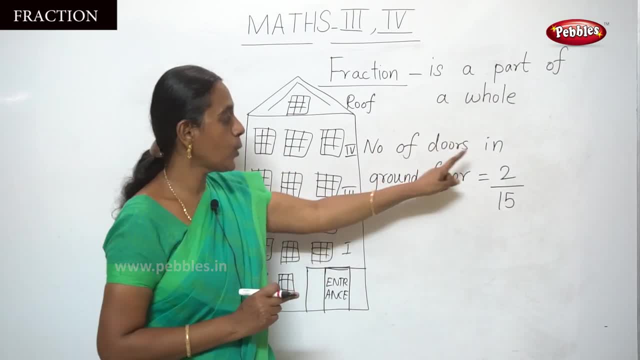 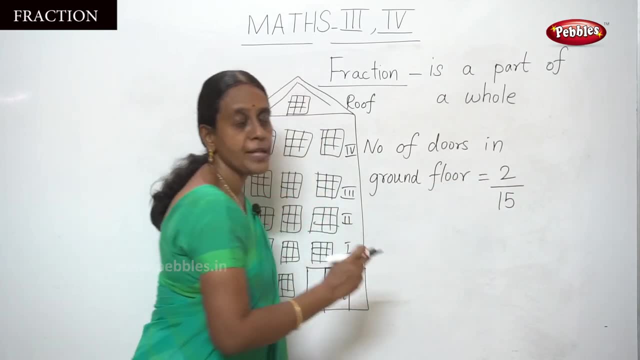 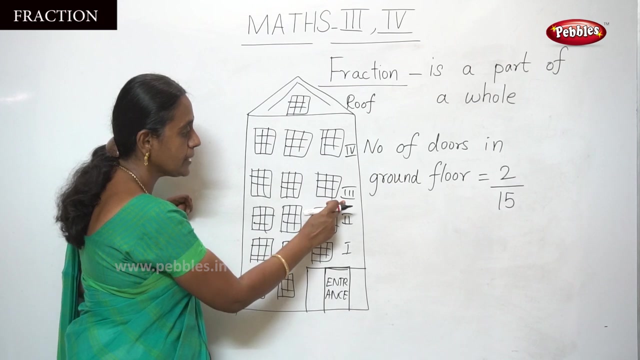 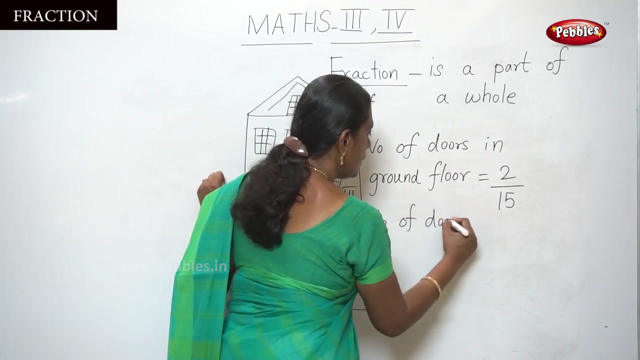 whole. okay, that is number of doors in ground floor means you have to count the doors in ground floor and this one is the 15, represents the whole part. that is a total number of windows. okay, and similar to that of here. that is a number of doors in third floor. number of doors in that is third floor. 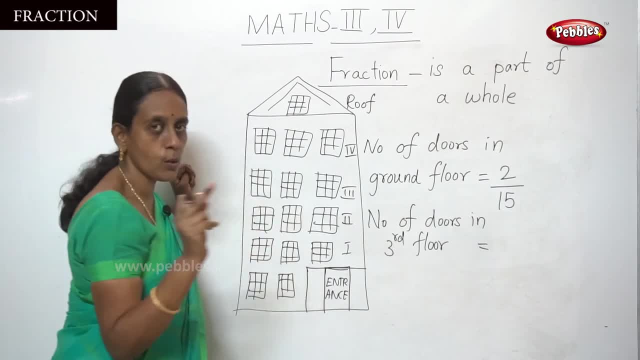 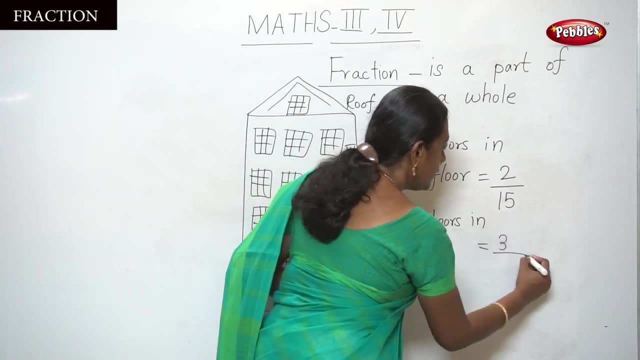 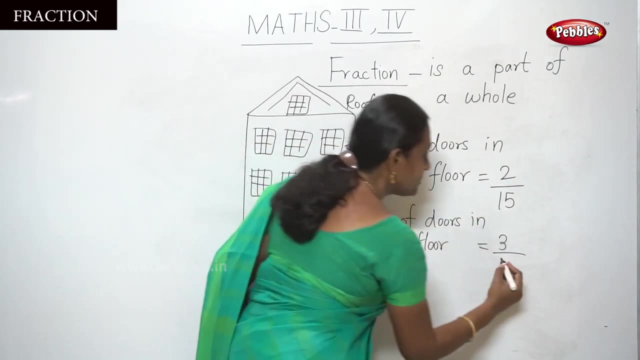 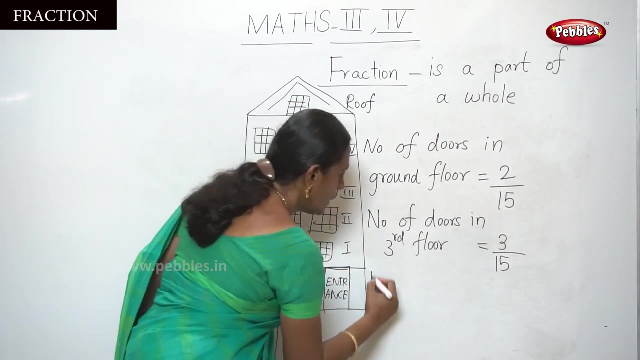 here, that is third floor, you have to count the door number of doors. that is 1, 2 and 3. okay, put the number 3 divided by the total number of doors. that is, we have already count. that is 15, okay, okay. and the number of doors in roof? okay, and that is number of doors in roof. 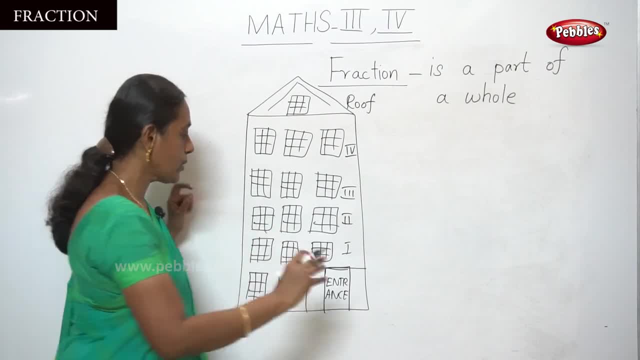 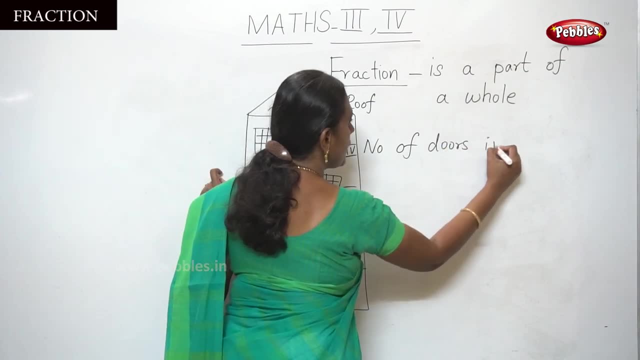 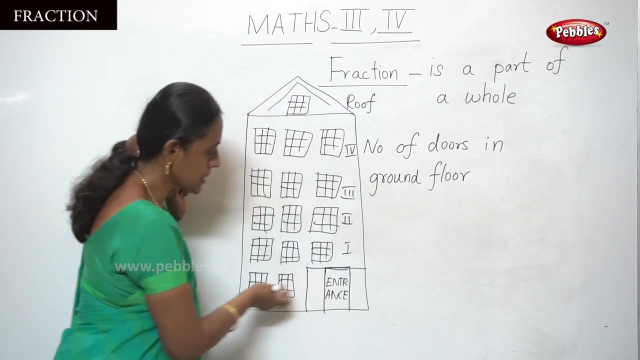 is ground floor, So you have to calculate. I'm going to write the question: Okay, number of doors in ground floor, Number of doors and ground floor. This is a ground floor, And how many times am I having to count this? Oh, close, Second. So here you have to count the door. 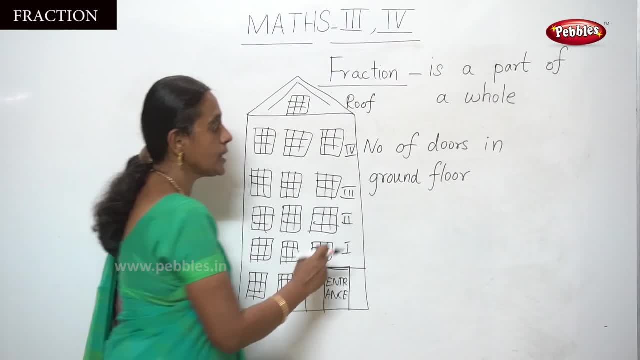 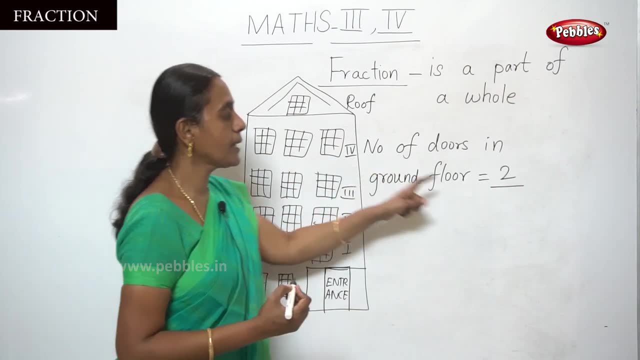 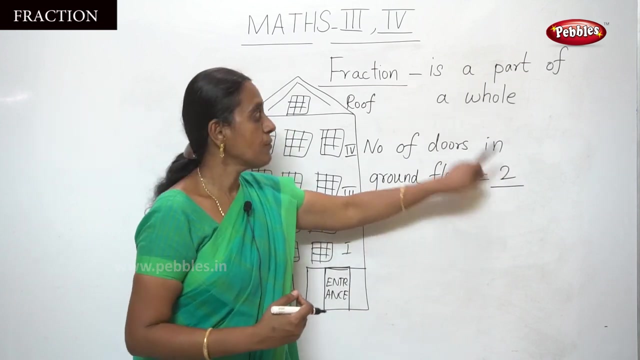 that is one and two. This one is the entrance door. these are the two doors, So that is number of doors in ground floor. That is two And fraction is all ways be like this: one number is we have to write in top and the other number, that is, should be written in below. So fraction. 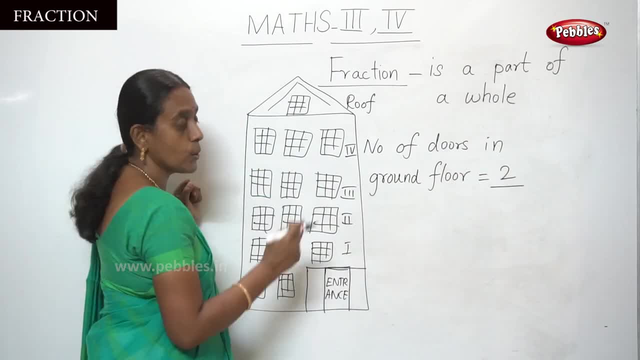 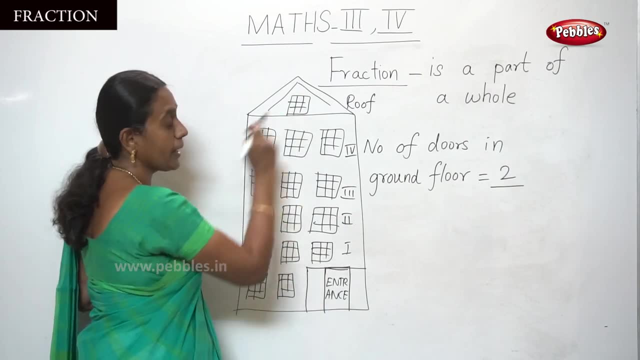 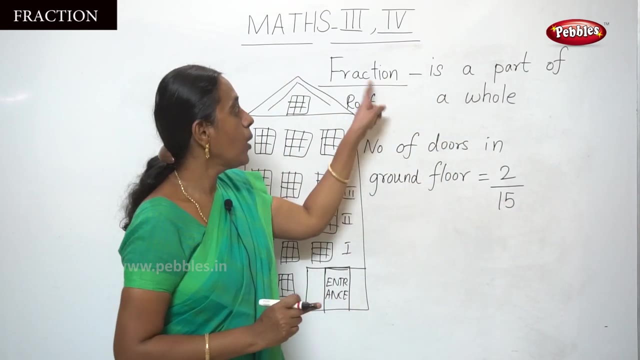 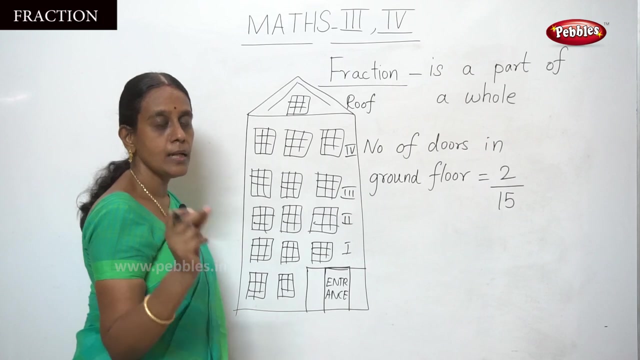 is like the two by and other number down. here that is all: 3, 6, 9, 12, 13, 14 and 15. here that is 15. this is a total portion that is called whole. okay, that is number of doors in ground floor means you have to count the doors in ground floor. 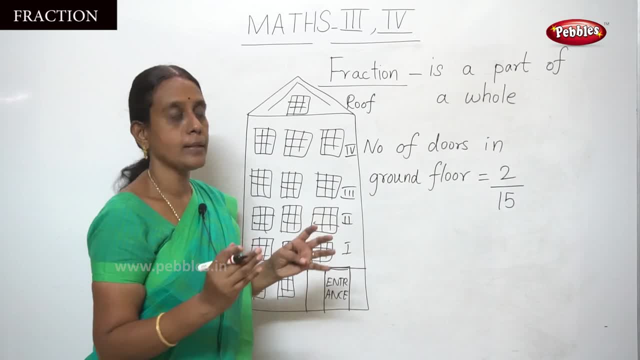 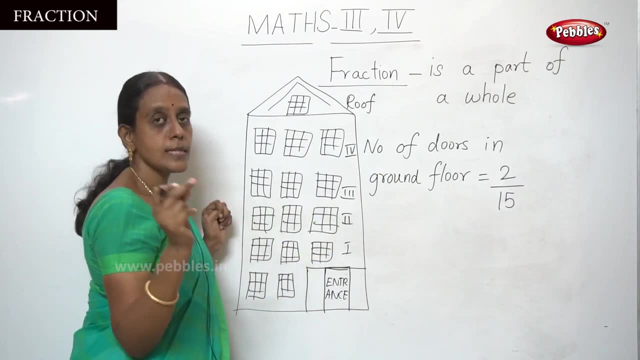 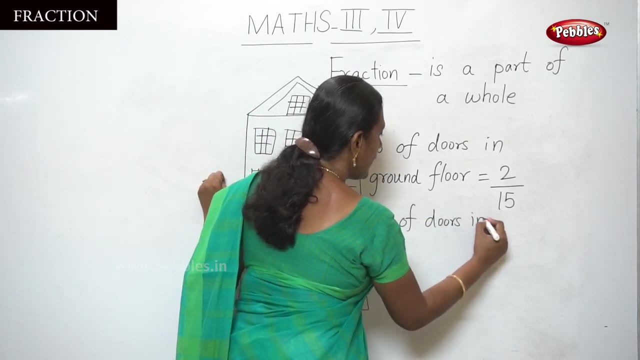 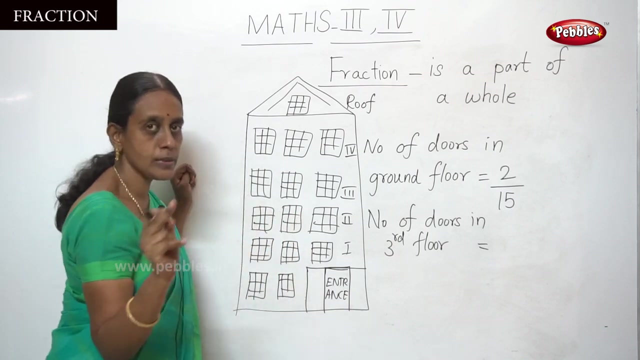 and this one is the 15, represents the whole part. that is a total number of windows. okay, and similar to that of here. that is a number of doors in third floor. number of doors in that is third floor. here that is third floor. you have to count the door. number of doors. that is 1, 2 and 3. okay, put. 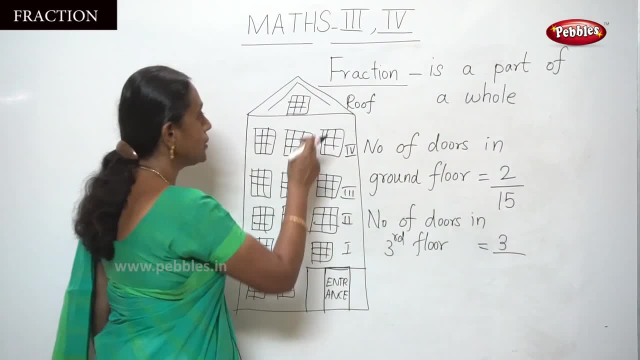 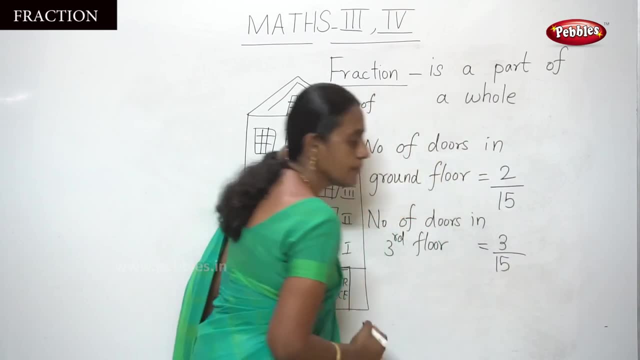 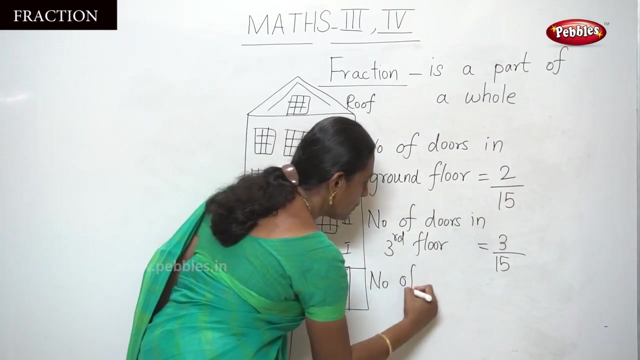 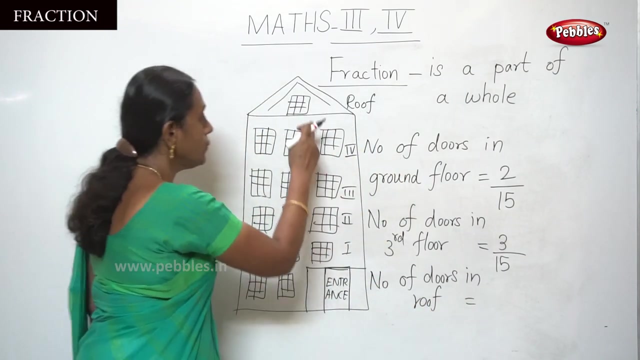 the number 3 divided by the total number of doors, that is, we have already count- that is 15, okay, okay, and the number of doors in roof: okay, and that is number of doors in roof. okay, here, the roof, the, there is only one door. okay, that is put one. and total number of. 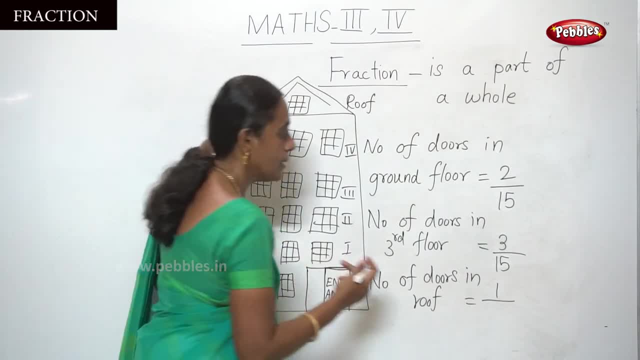 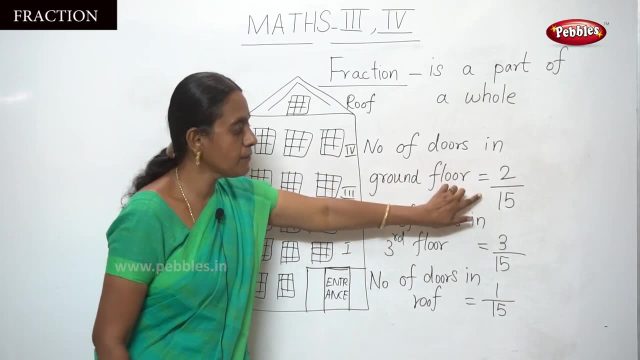 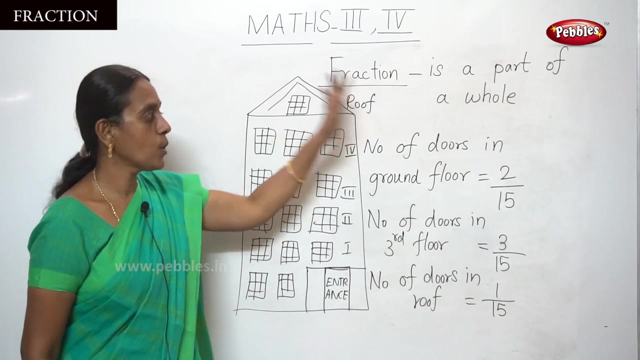 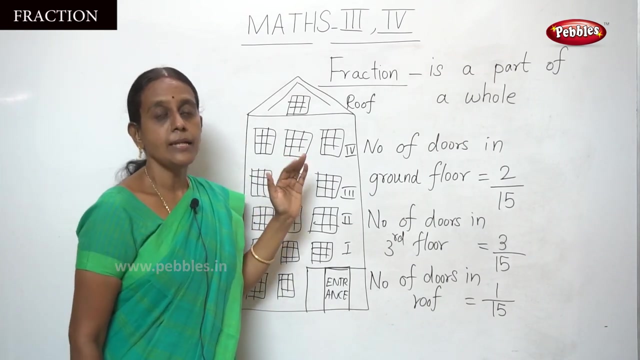 windows, that is doors, that is. we have counted that is 15. so this answers that is 2 by 15 and that is 3 by 15 and 1 by 15. these are. that is called as fraction. okay, do you understand? now that is a similar to that of our division. in division topic we have 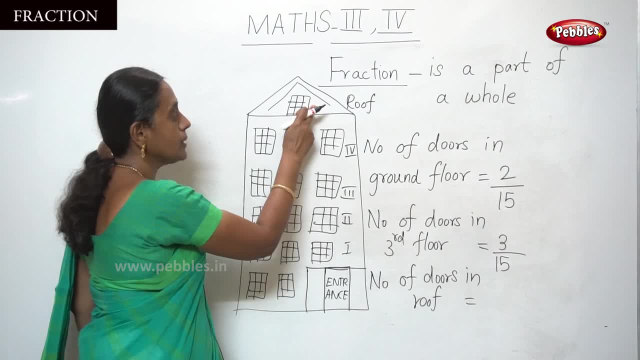 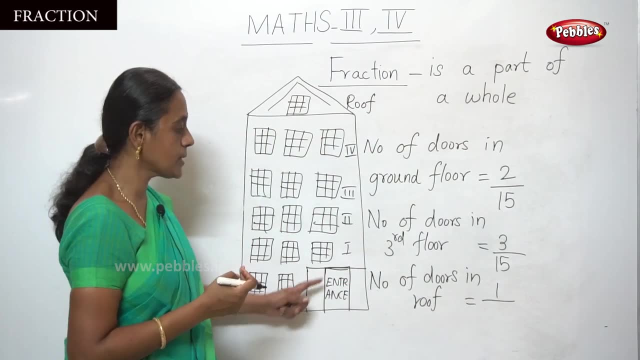 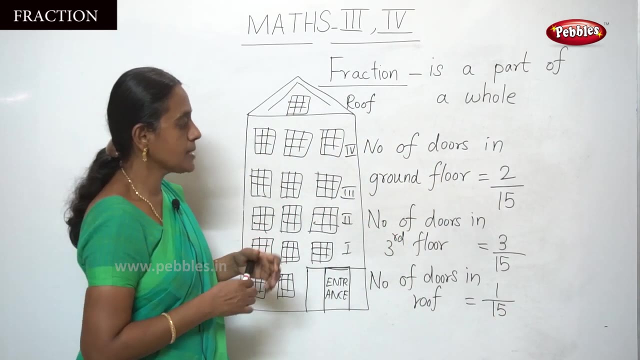 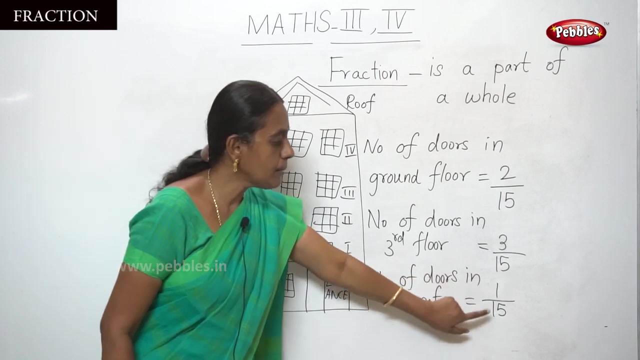 okay, here the roof, the, there is only one door. okay, that is put one, and total number of windows: there is doors: that is, we have counted, that is 15. so this answers that is 2 by 15 and that is 3 by 15 and 1 by 15. these are: that is called as fraction. 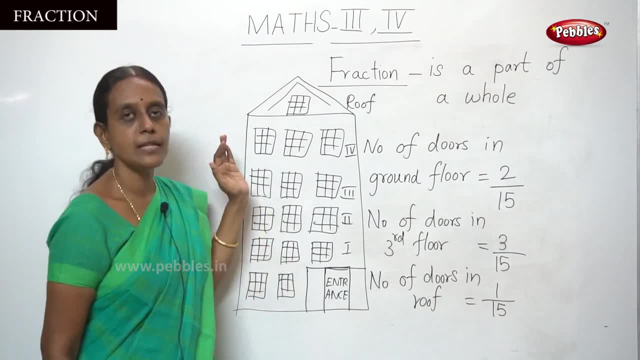 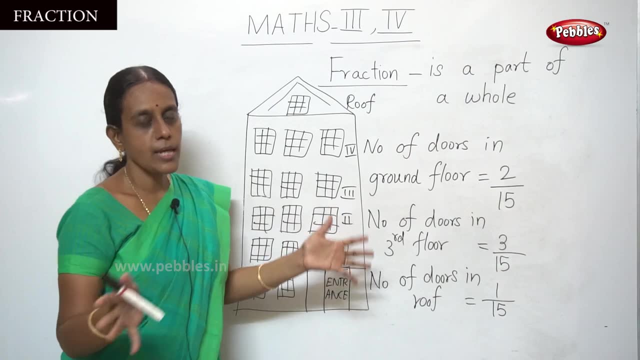 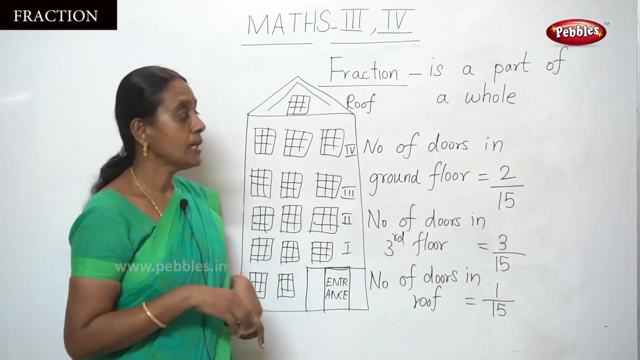 okay, do you understand? now that is a similar to that of our division. in division topic we have to divide the materials or everything to the among the equal share to the people's or content. okay, that is division, and counting of cost of one, that is division here. 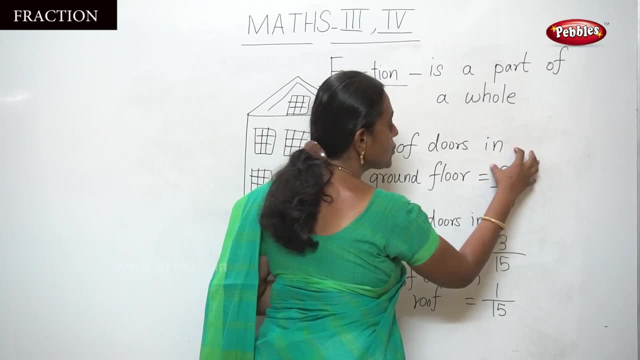 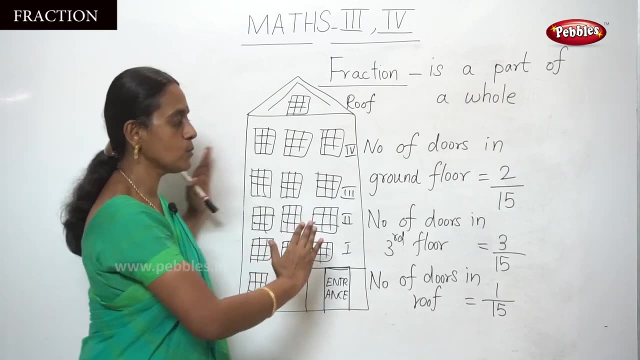 so that is what I tell you. or that is what I tell you is to divide and count those, all the things, that is, each Mmm fraction and the whole number block. I am also talking about a section, So this sheet is my group table, easy to be aware that each one of them is my list. 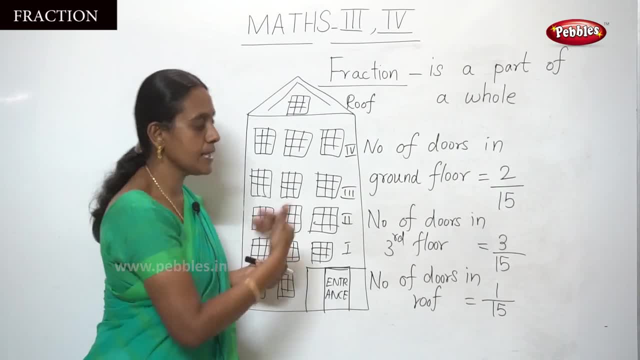 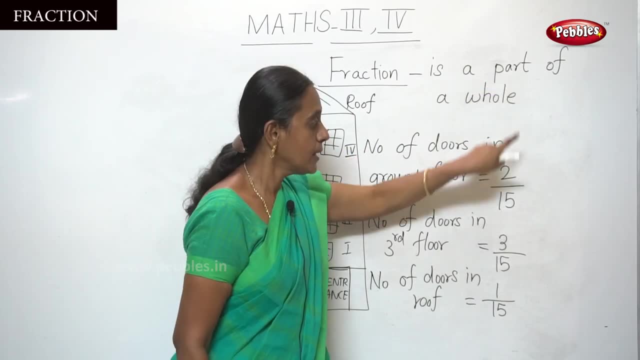 mother part fourth fifth and as you will notice I have this section Nazgan in the fifth column the first left and the second one has a section name number two. so today we have that is from this whole number block to � wa n it is second number that needs to be a should I more simple and simple just like I already applied to for this in another table ok. 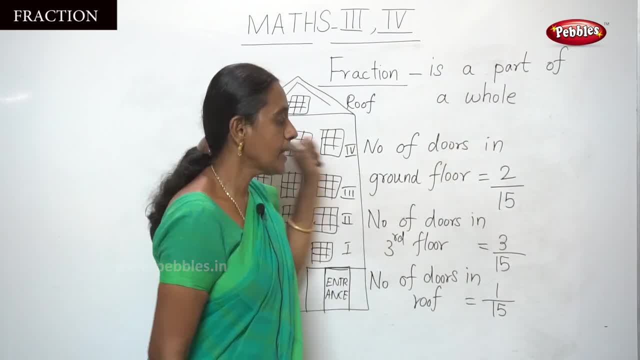 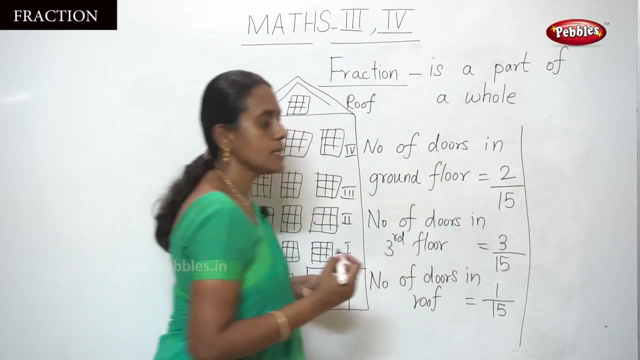 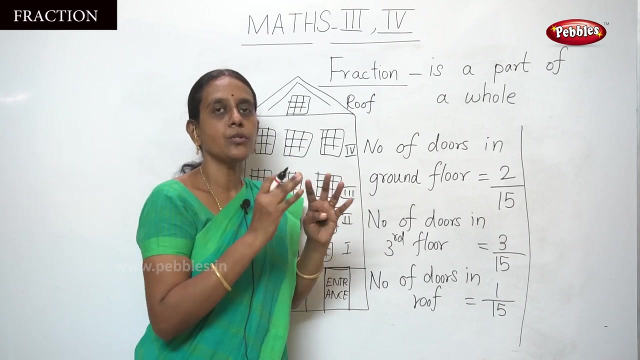 15. number of 15 is the whole. okay. and one more example for your reference. suppose yours mom- okay, uh, that is about one pizza or one, make it as one doza. two, that is one doza you have. yours mom is going to divide into three persons. okay, simply, this is a doza. okay, this is a doza. 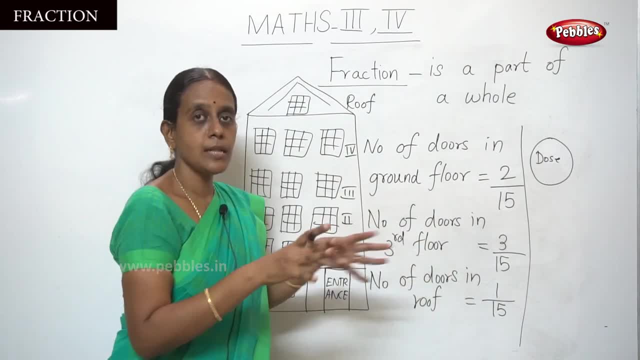 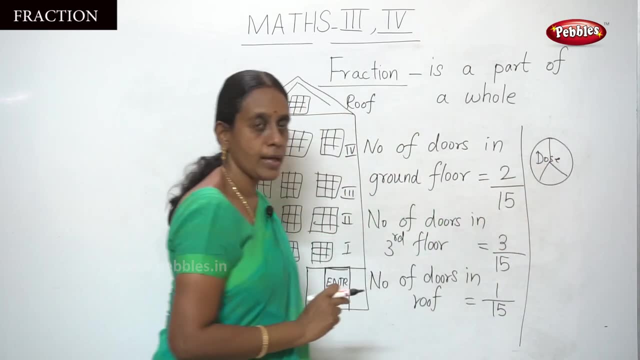 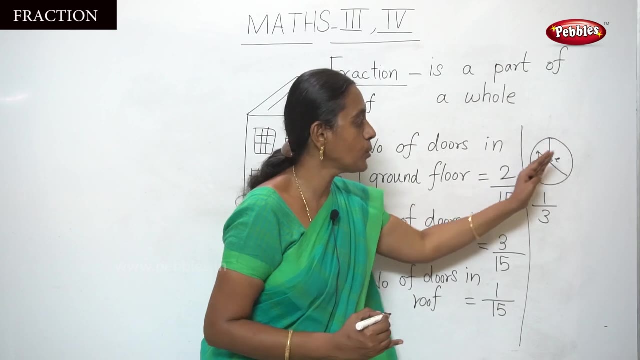 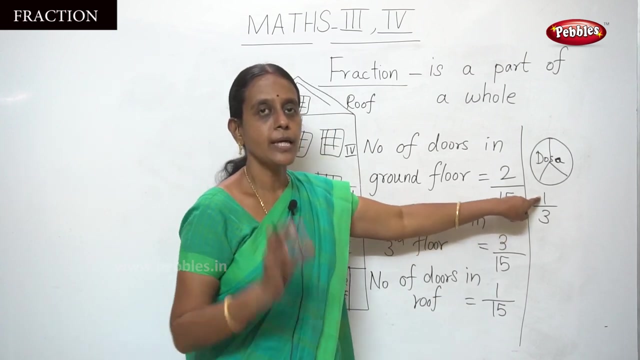 okay, yours mom going to divide this three persons. that means okay, like this: okay, one, two, three. okay, that is one two, three, that is one by three. so each person has one portion of this doza. so this is a fraction, so one is a portion of each one get and three is a total number of whole part. 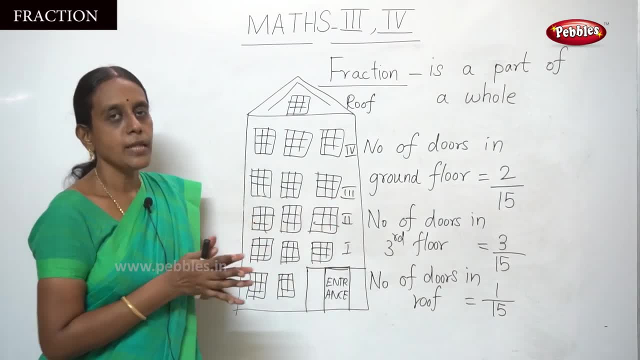 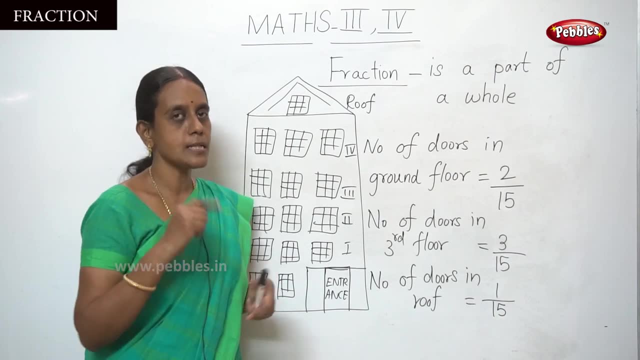 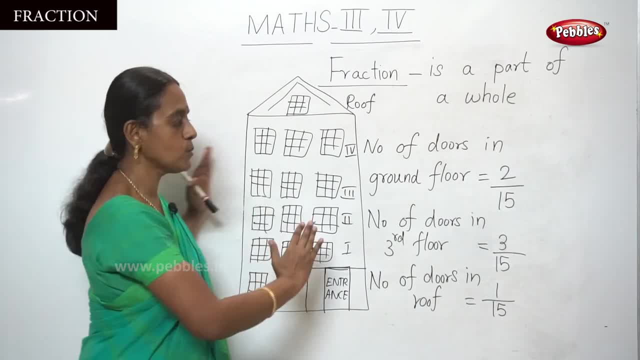 okay, so we have to divide the materials or everything to the among the equal share to the people's or content. okay, so we have to divide the materials or everything to the among the equal share to the people's or content. fraction. next we are. that is what is meant by fraction, and next we move on to the. that is, terms. 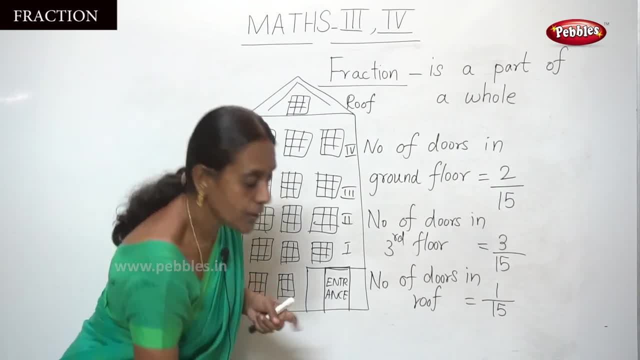 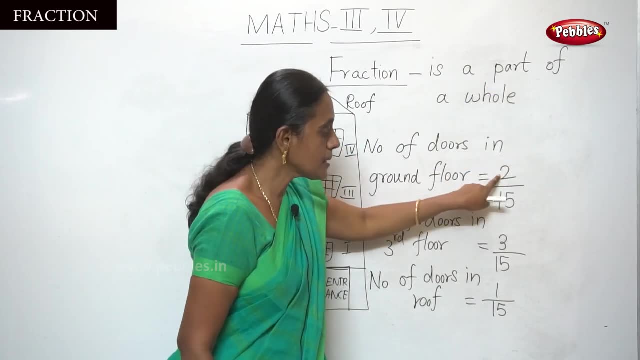 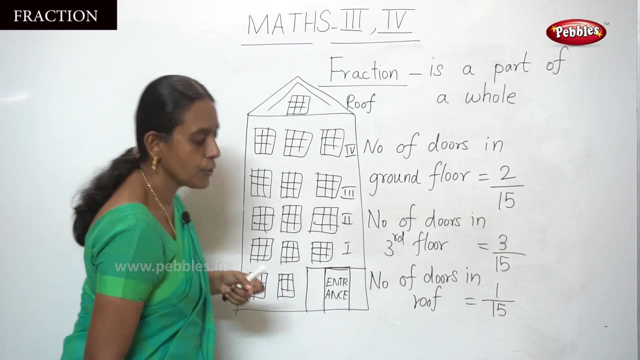 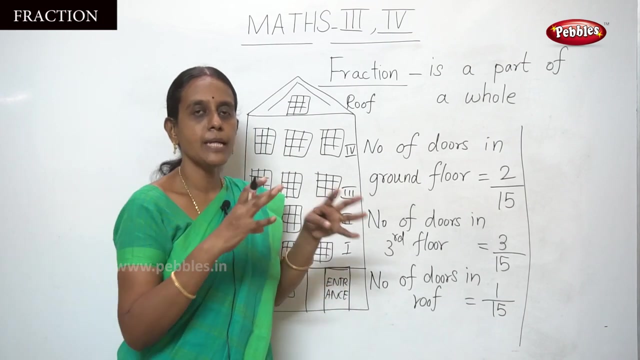 what are the terms used in fraction? let me see. okay, do you understand this? that is what is meant by whole and what is meant by part. okay, this is a part and the 15 number of 15 is the whole. okay, and one more example for your reference. suppose yours mom. okay, that is about one pisa or one make. 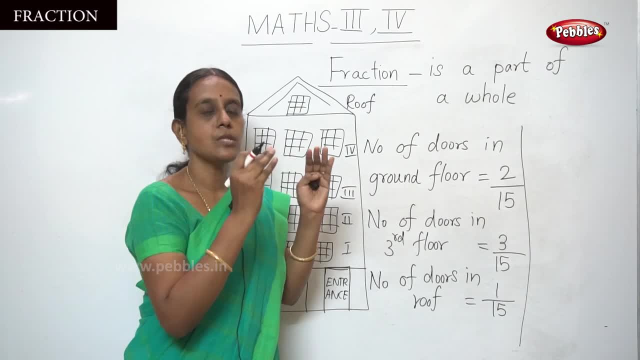 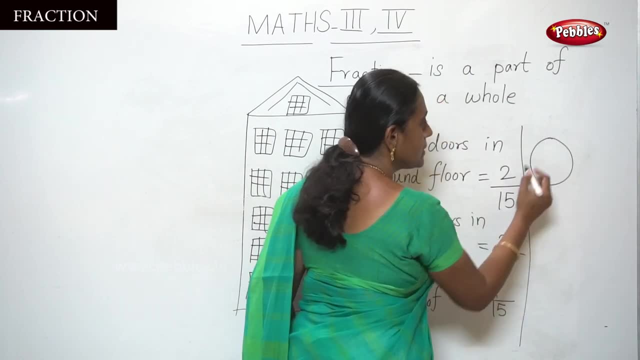 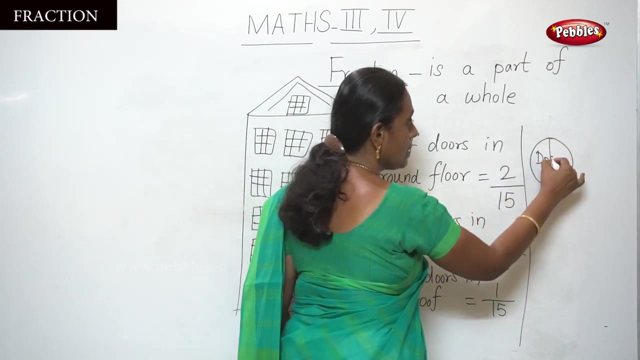 it as one doza to. that is one doza you have. yours mom is going to divide into three persons. okay, simply, this is a doza. okay, this is a doza. okay, yours mom going to divide this three persons. that means, okay, like this. okay, one two. 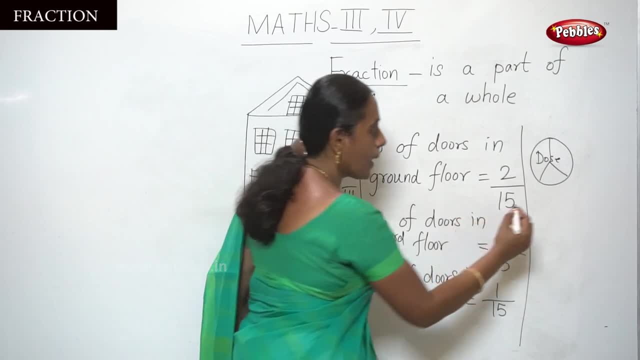 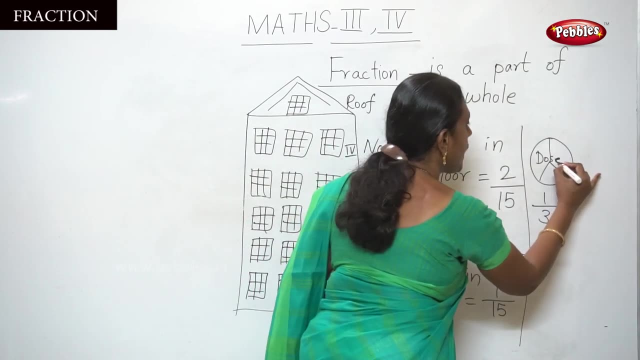 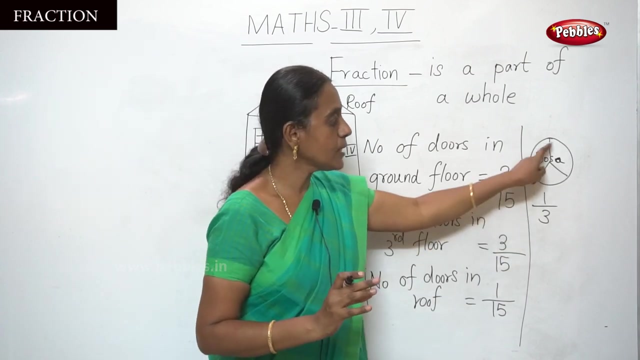 3. okay, that is 1, 2, 3, that is 1 by 3. so each person has one portion of this dosa. so this is a fraction, so 1 is a portion of each one get and 3 is a total number of whole part. okay, and let me. 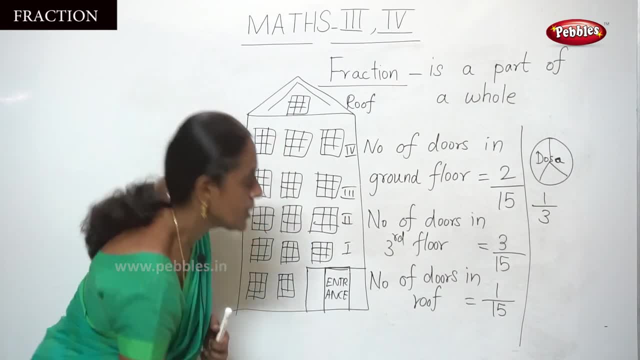 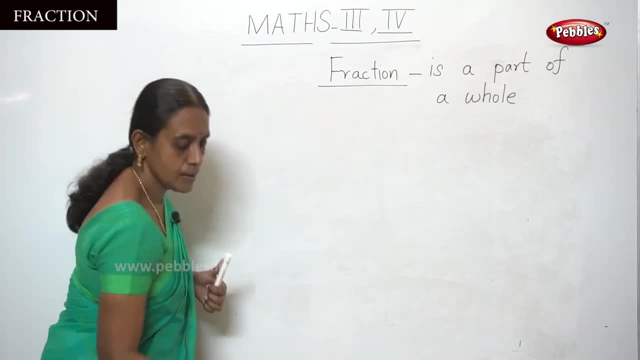 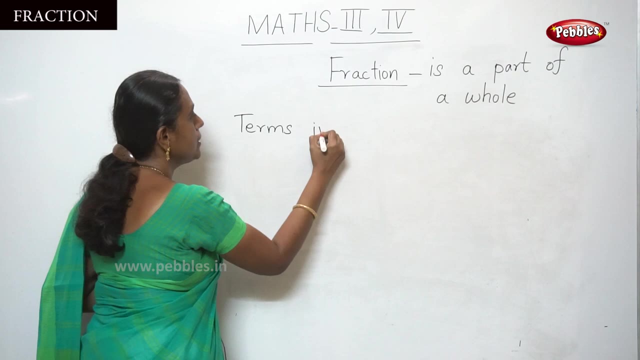 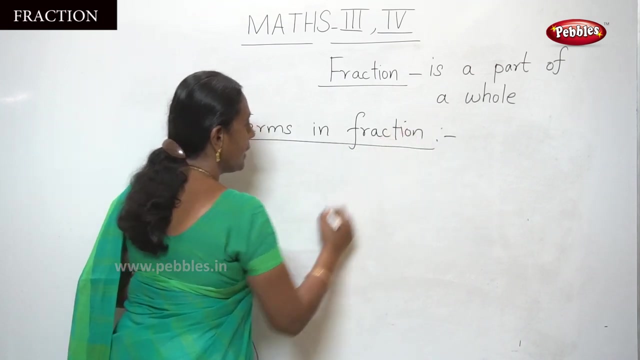 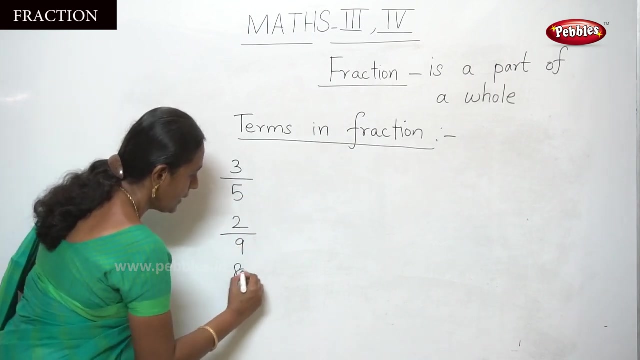 move on to the next, that is terms in fraction. okay, i'm going to write with example this: that is fraction, we have learned the definition. and next, that is terms: terms in fraction. okay, and that is 3 by 5, 2 by 9, 8 by 11. okay, these are the few examples of 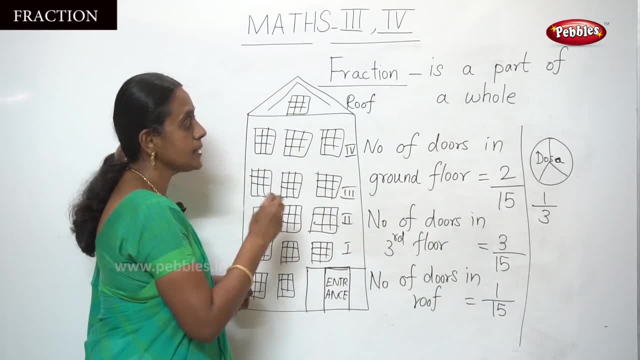 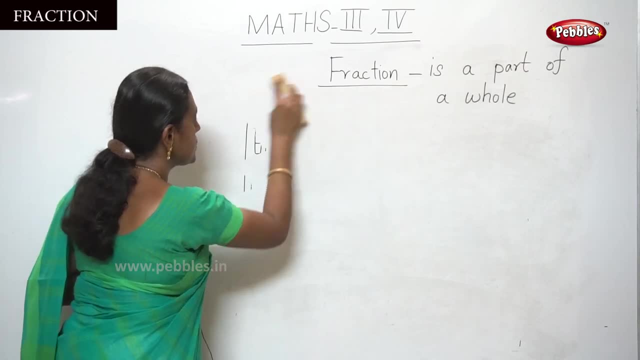 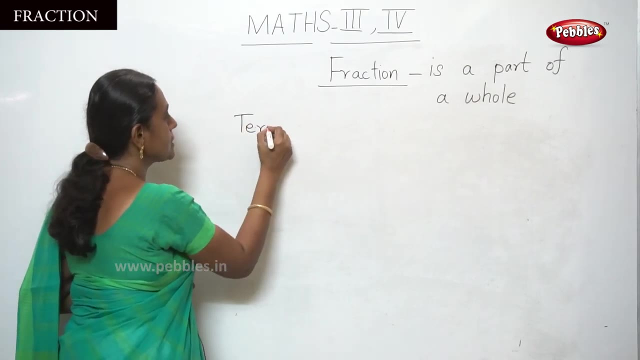 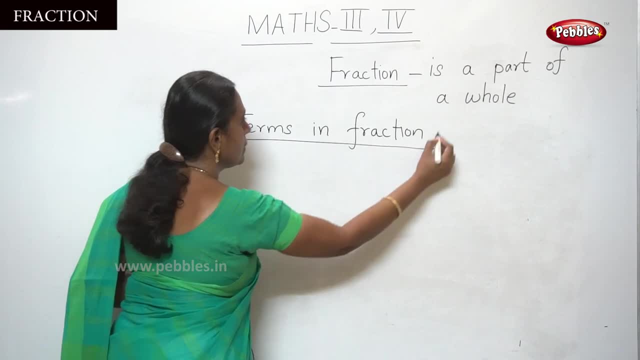 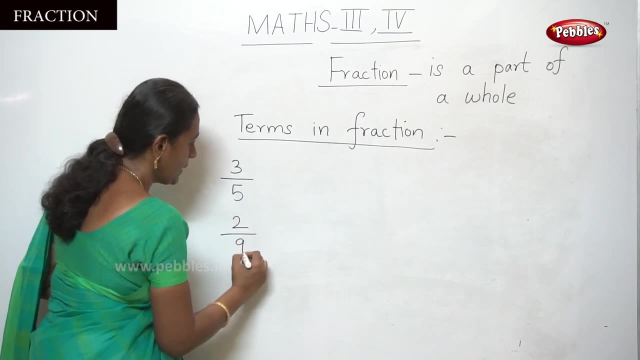 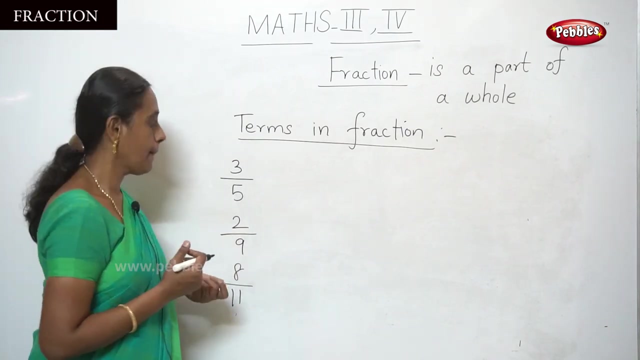 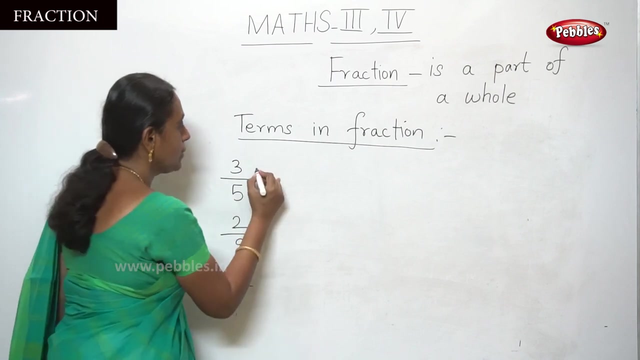 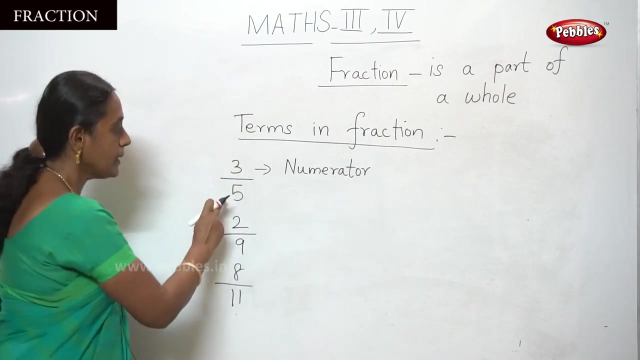 okay, and that is three by five, two, okay, okay. by nine. eight by eleven- okay, these are the few examples of fraction. now that is the number that is written as the top is called numerator okay. which one is called that is numerator okay? and the lower bottom one, written in the bottom portion, that is a denominator. 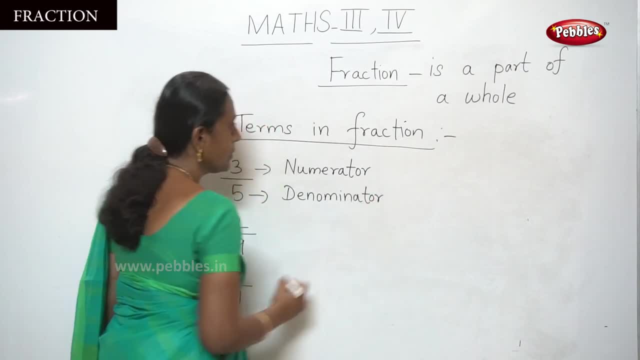 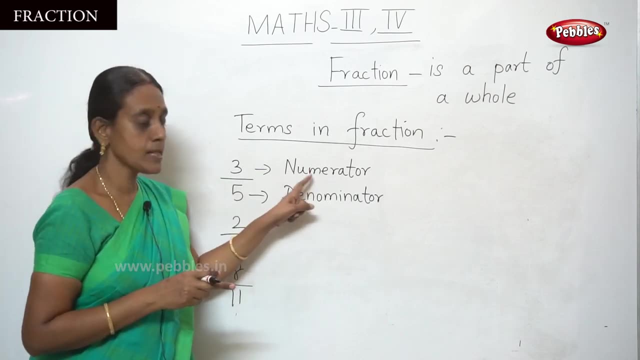 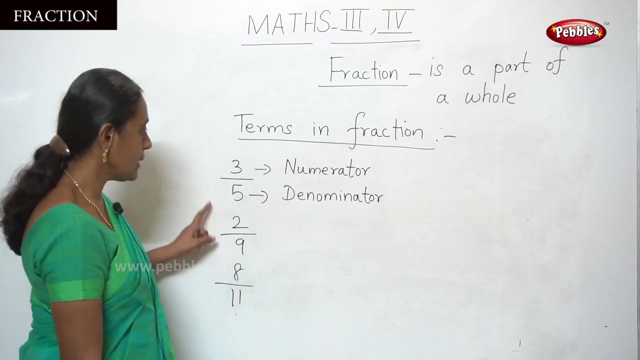 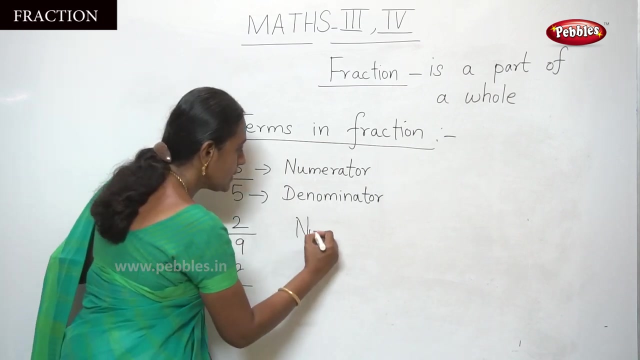 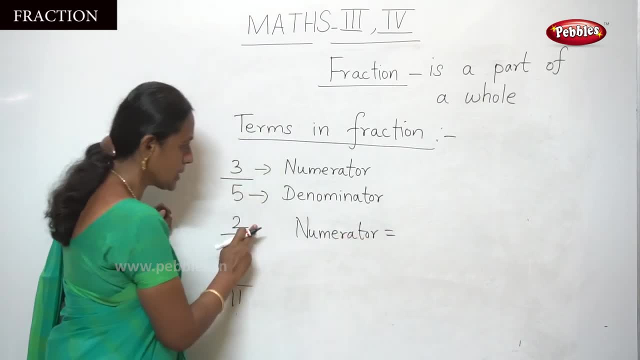 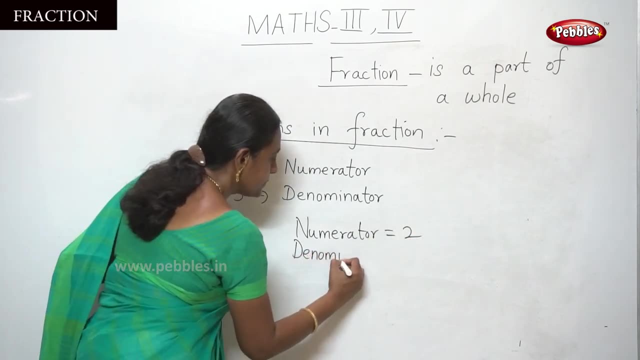 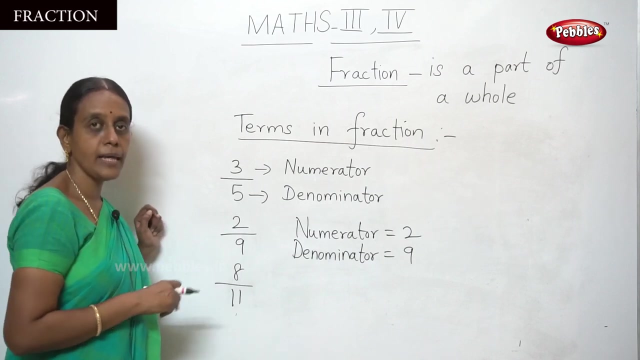 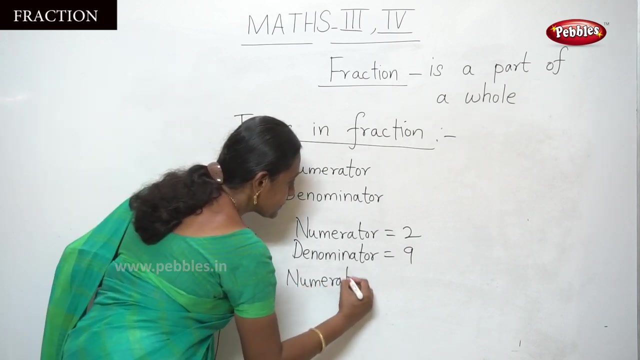 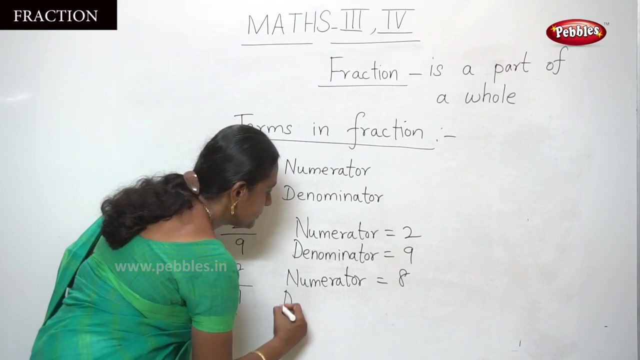 okay, write this answer for this: numerator here that is two, 2, and the denominator that is 9,. denominator that is 9,. okay, and that is 8 by 11,. okay, 8 by 11,. here the numerator is that is 8 and the denominator is 11, is 11, okay. 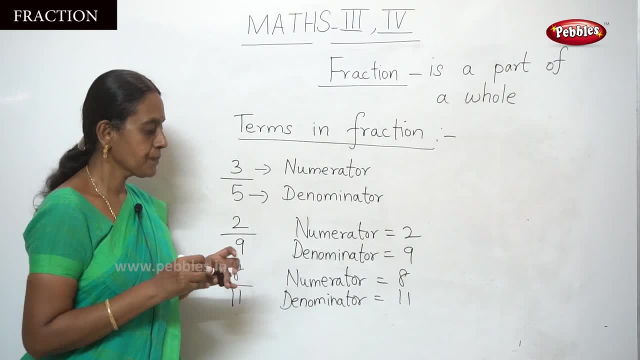 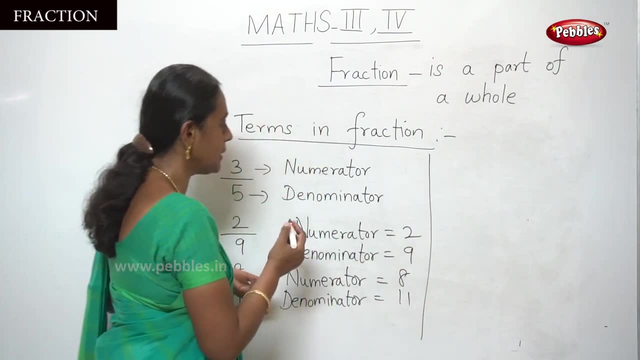 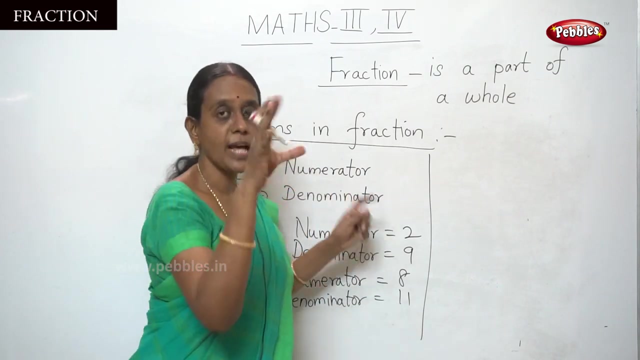 So this is a. these are the terms in fraction. which is meant by that is numerator and denominator for your exercise sums. The question will be that The numerator and denominator is given. So you asked to write: that is the fraction. You are going to write the fraction in your question that the numerator and denominator.